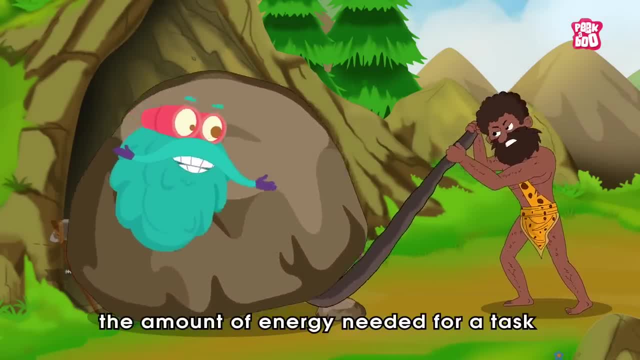 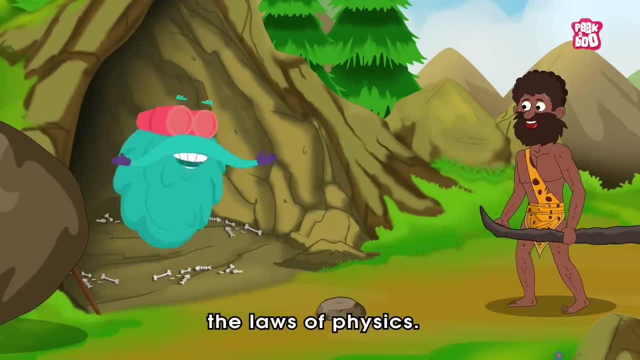 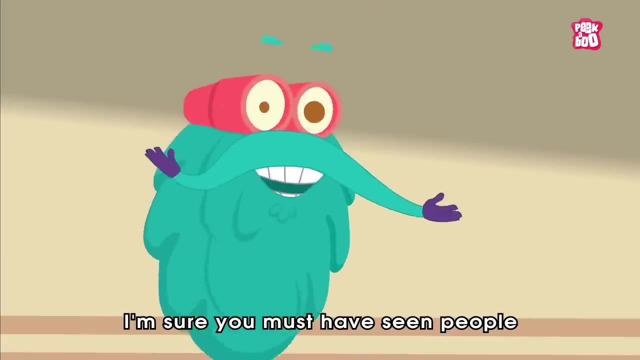 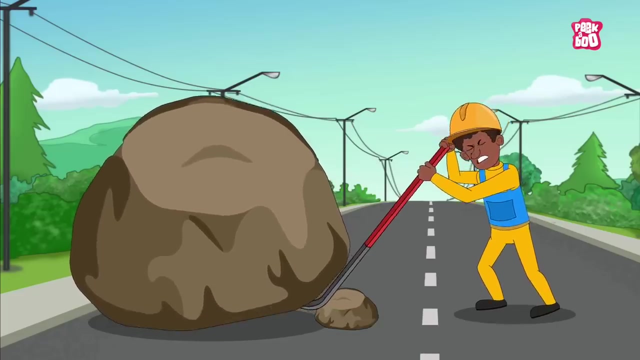 These machines helped reduce the amount of energy needed for a task and multiply the force by cleverly applying the laws of physics. How, Let me explain them. starting with this, A simple machine can move a heavy object with the lever. I'm sure you must have seen people using a crowbar to move a heavy object like a rock or a log. 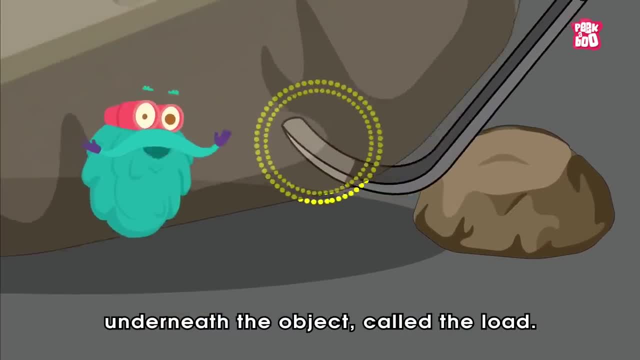 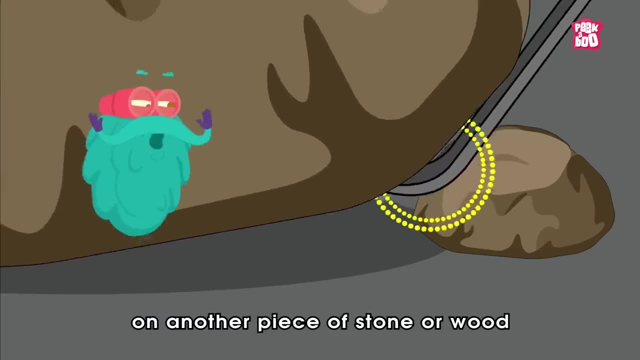 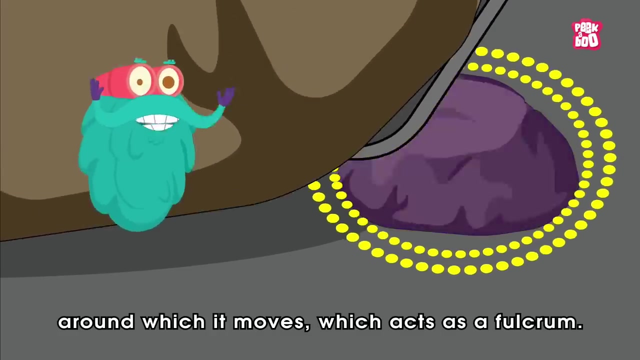 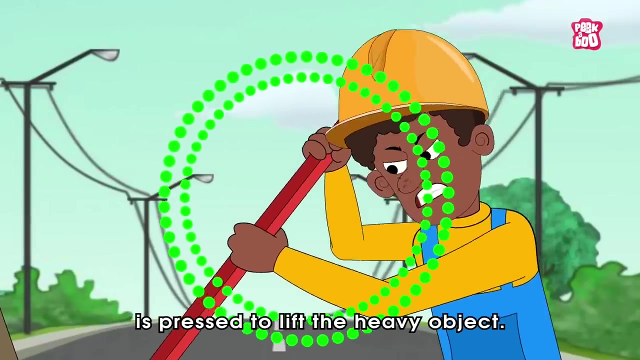 The end of the crowbar is placed underneath the object called the load, Whereas some part of it is made to rest on another piece of stone or wood around which it moves, which acts as a fulcrum. Then the free end, also known as the effort arm, is pressed to lift the heavy object. 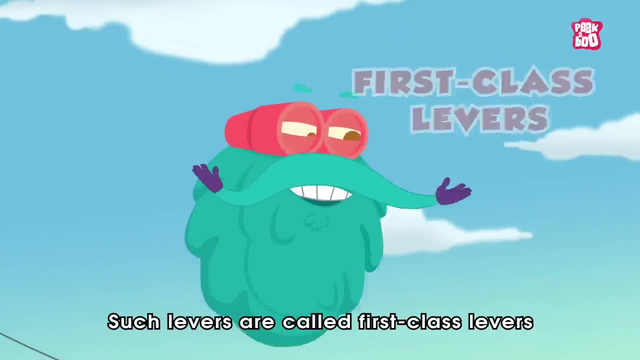 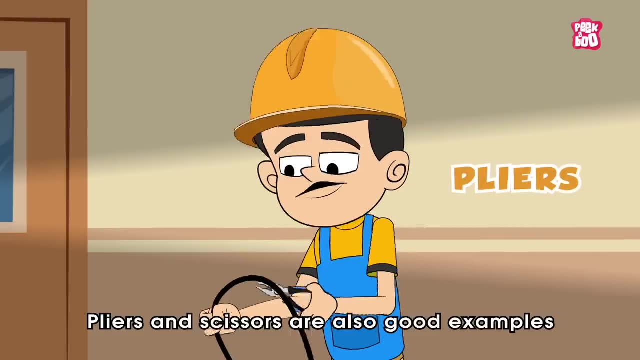 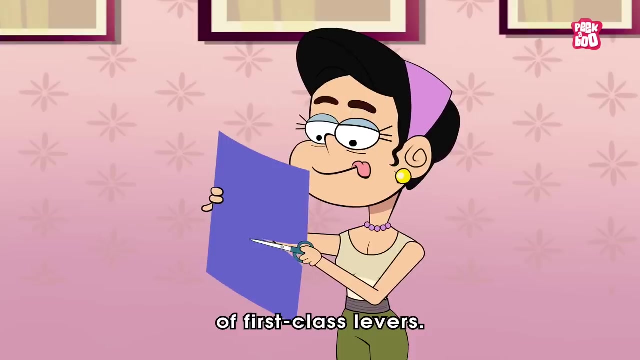 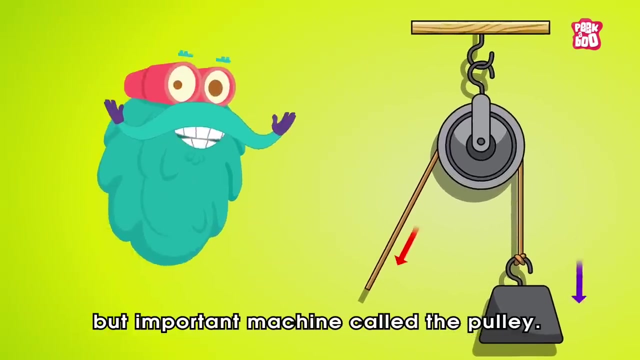 Such levers are called first class levers, where the fulcrum is kept between the heavy object and the effort. Pliers and scissors are also good examples of first class levers. Now let's look at the next simple but important machine called the pulley. 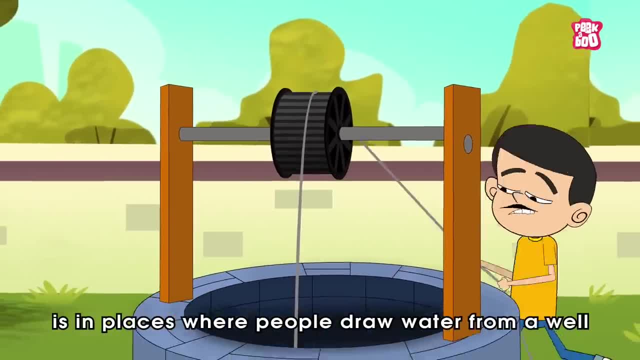 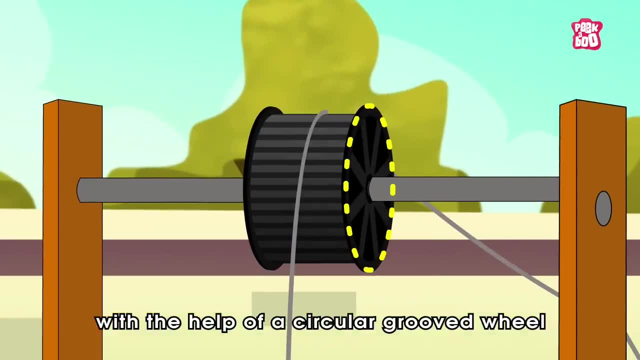 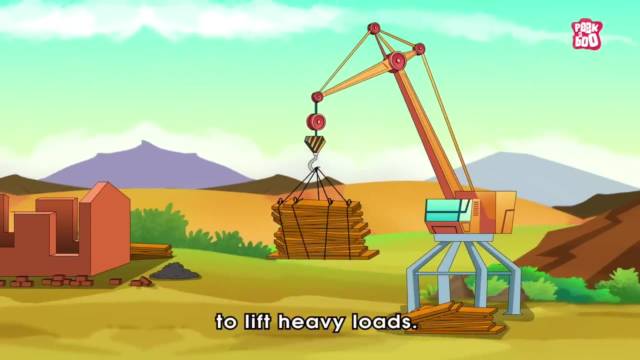 A good place to see this mechanism working is in places where people draw water from a well with the help of a circular grooved wheel over which a rope runs. Similar techniques are used in cranes to lift heavy loads. Have you ever seen a screw that helps to join things? 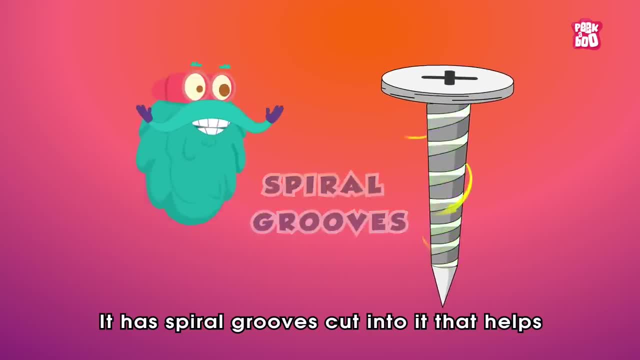 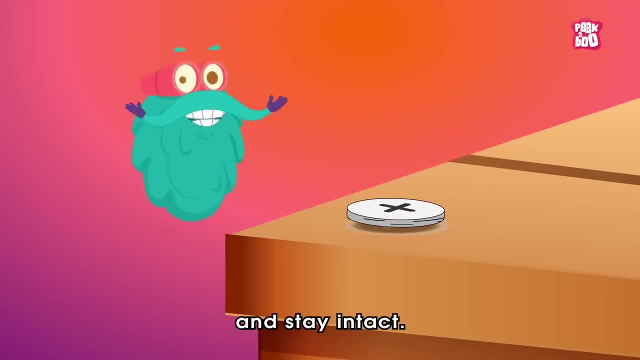 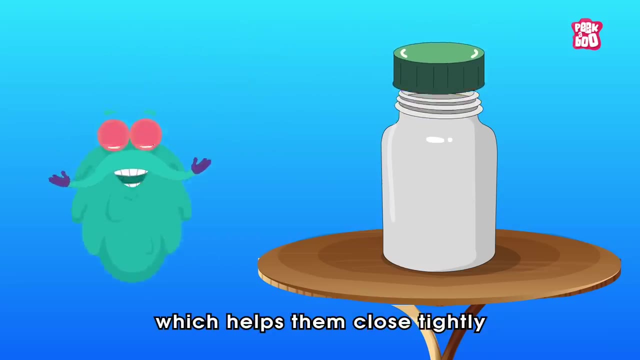 Let me show you. It has spiral grooves cut into it. that helps the screw easily go inside any surface and stay intact. The same mechanism is molded on bottle caps and tops of bottles, which helps them close tightly. The next simple machine looks familiar. 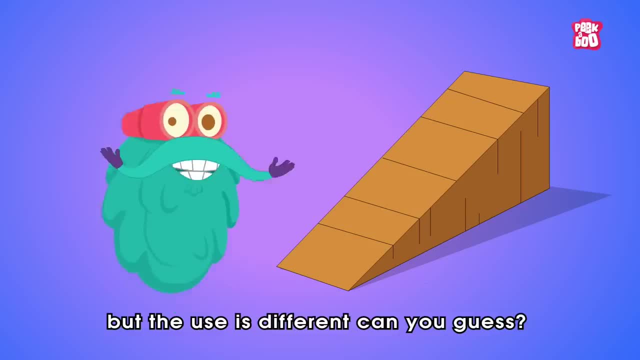 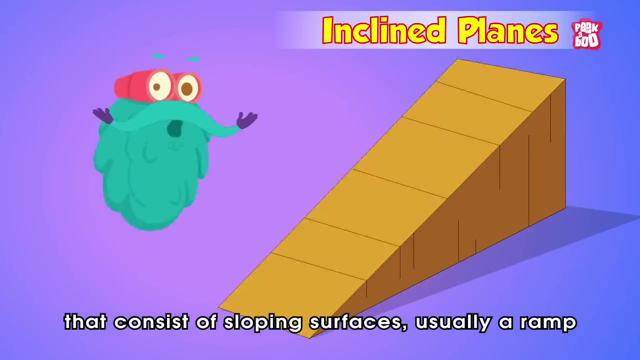 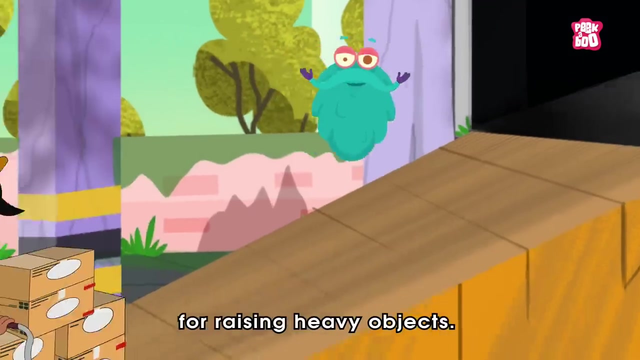 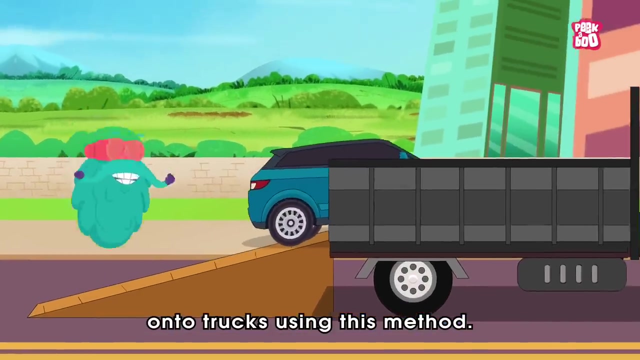 But the use is different. Can you guess? Okay, got you covered, my friends. In blind planes that consists of sloping surfaces, usually a ramp set at an angle against a horizontal surface for raising heavy objects. You must have seen cars being loaded onto trucks using this method.